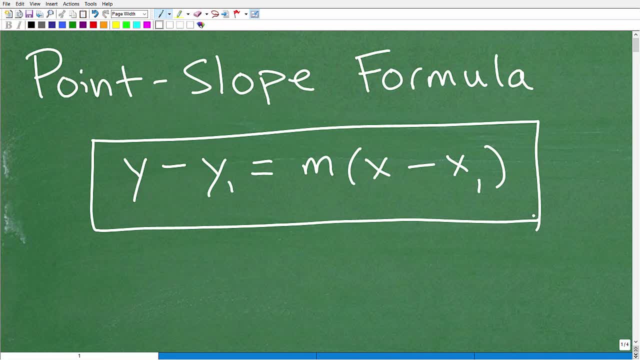 course, I'm going to leave a link to my math learning program in the description of this video. You can check out my full courses there And, if you like my teaching style, I'd also encourage you to subscribe to my YouTube channel. So I'm posting stuff all the time. I already have hundreds and hundreds of math videos there for you And, of course, if you enjoy this video and get something out of it, please can consider smashing that like button. Okay, so let's get to it. Point-slope formula. All right, what are we talking about here? Well, let me just kind of 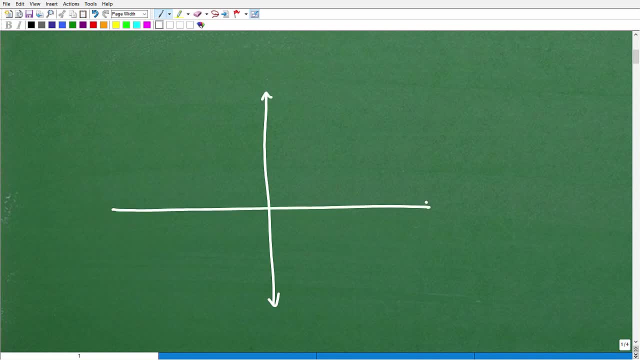 draw a quick x- y axis here, All right. so let's just use an abbreviation- point-slope formula, All right. what is the deal here? Well, the deal is this: Okay, we're talking about linear equations, all right, which are lines like so, Okay, And we're trying to find the equation of some line? All right, this is like you know. think of yourself as a detective. We're trying to find the. 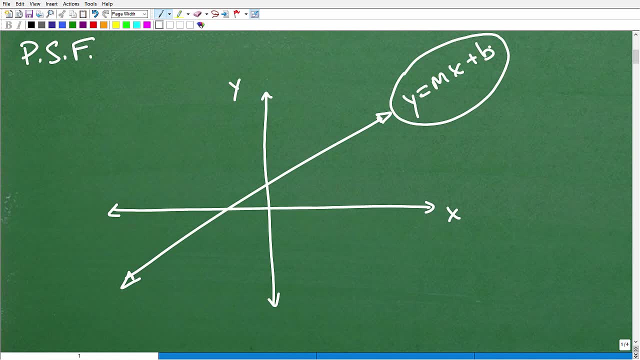 equation And more often than not, we're trying to write this equation in: y equals mx plus b, form right. So in other words, for example, this line might have an equation of y equals 2x plus 1.. Okay, so we're trying to find the equation, what we call the linear equation. This is an equation. 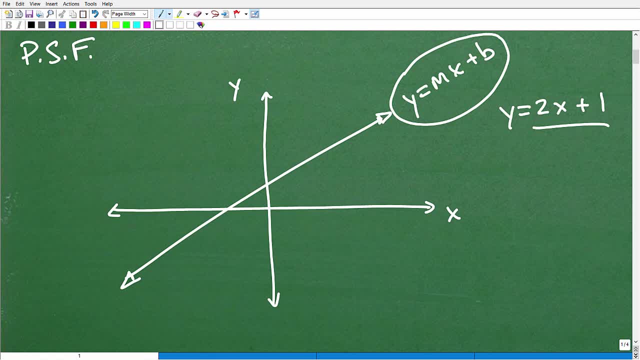 that models this line. Okay, so this is what we're trying to do, And the point-slope formula allows us to do this, But we need to have some other basic, fundamental things about finding the equation of a line. Okay, so we're trying to find the equation of a line. 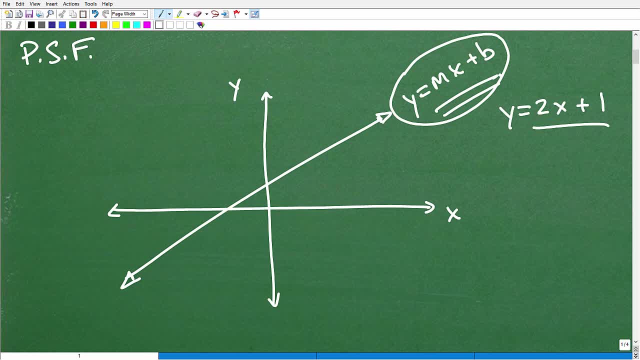 What do you need to find the equation of a line? Well, you need the slope. Okay m, All, right, slope. And by the way, I'm assuming you have some background already with the slope and graphing lines, etc. If you don't, you know, if you're not familiar with what the slope is or how to graph a. 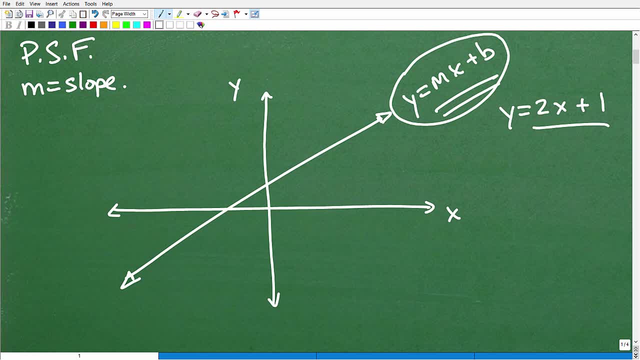 line, then you know you might want to go back and review, Because that's kind of a prerequisite before you get into this stuff. All right, so we need the slope, all right, of a line that we're trying to find out. So, for example, this line: we're saying: 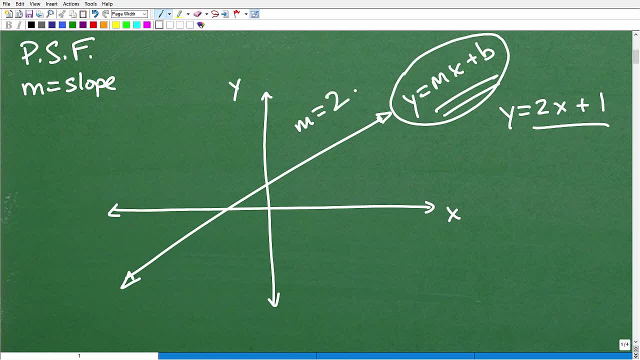 okay, the slope is, let's say, 2.. And we also need to know one point. okay, at least one point that's on that line. So if I say, hey, I have a line, its slope is 2, and the point, let's say this point. 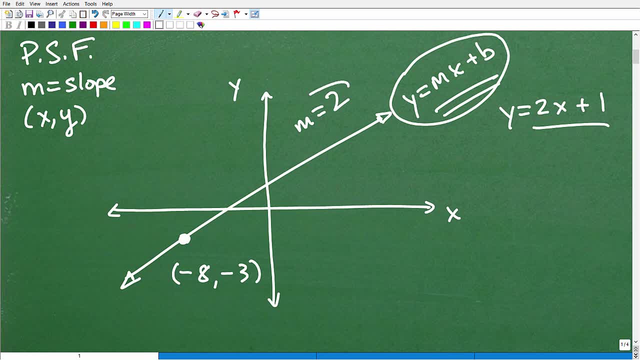 3,. okay, this point is on this line. I know the slope of this line. That's all the information you need to find the equation of a line. Now you have kind of two options here. right, You can take the point slope equation. Let me just write this here And this is what we're going. 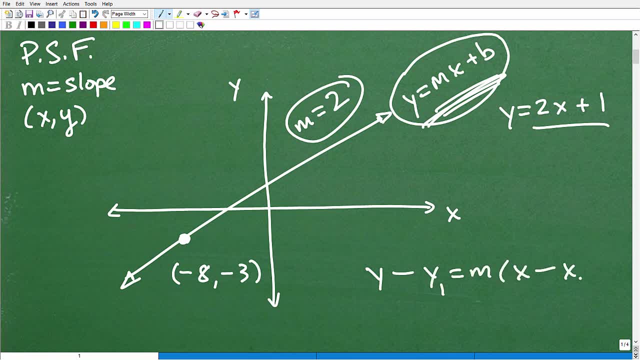 to focus on in this video. All right, I love this equation. I think this is, more often than not, the primary way. I think that suits should, a primary formula that students should take when they're trying to find the equation of a line. 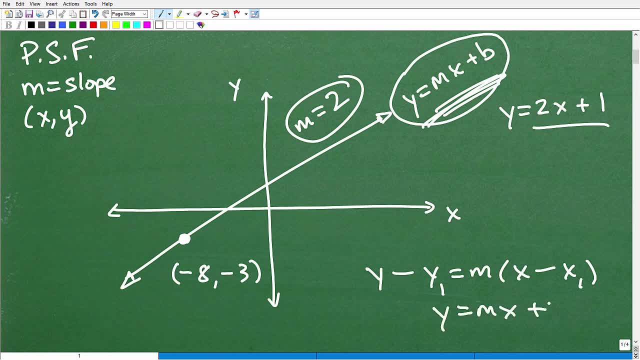 Or you can use y equals mx plus b and work with this slope intercept formula. Both are good. I prefer this method. This is what I kind of really focus on when I'm teaching- because it kind of just handles all situations very nicely. But either one of these formulas will get you your final. 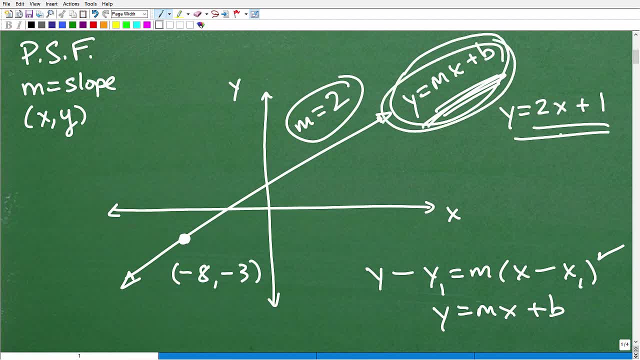 answer which will look something like this: okay, Now a couple things here. right, You need a plot, You need a point and the slope of a line. But let's talk about a situation real quick And I'm going to actually apply the point slope formula. What if we said, oh, we don't have the slope. 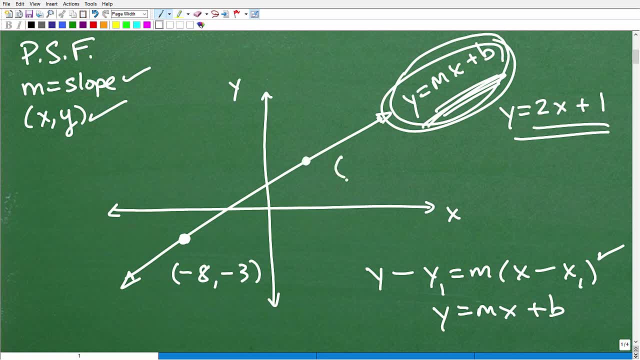 but I have another point that's on this line. So let's say, this point here is 2, 3, okay, So the question is: find the equation of a line. In other words, we want to find this: y equals mx plus b. 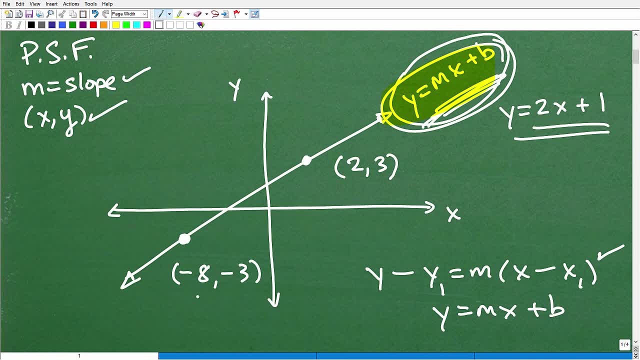 business. okay, Find the equation of a line, given that this line passes through these two points. okay, Negative 8, 3 and negative 8, 3, or negative 8, negative 3,, excuse me- and 2, 3, okay, So this line is passing through these two points. This is also fine, So. 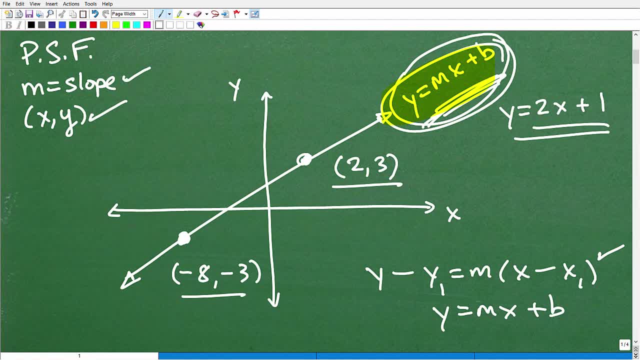 when you're trying to find the equation of a line, you need the slope and a point. That's what you need. But here I'm like: oh well, I got two points. Well, guess what Between these two points? 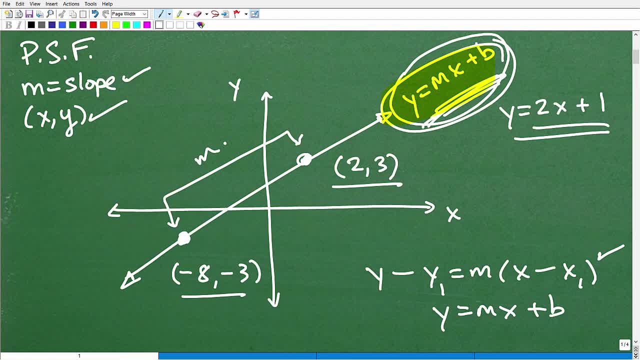 you can calculate the slope m, all right. So you need to know how to find the slope, given two points, okay. And then, once you have the slope, you need to find the slope and you need to find the slope. okay, You have the slope and you're like, okay, I need the slope and a point. Well, I have. 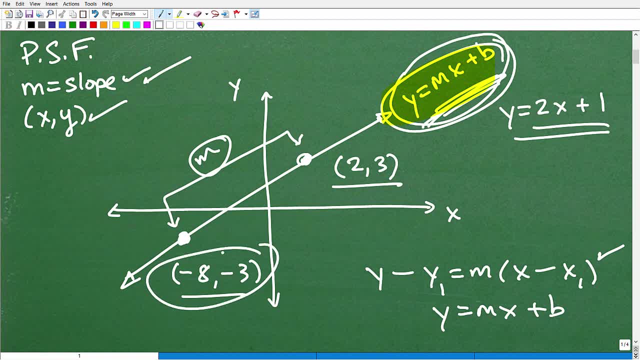 two points. Well, you can use either one and still get the right answer. You can use this point, or you can use that point. The slope is still the same, and then you can obviously get the right answer. All right. so I find, as a math teacher, that sometimes you know, students are confused. 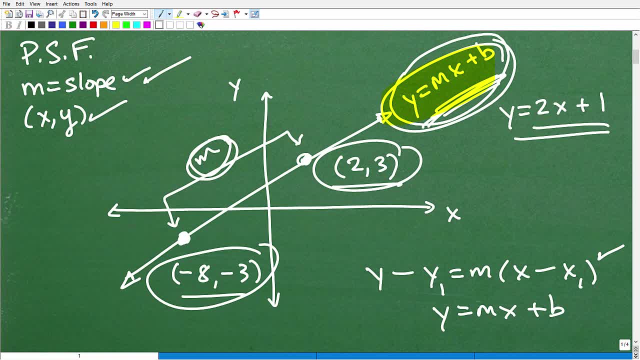 about? what is the formula about? What are we even trying to do? So this is an overview of finding the equation to lines. okay, Whether you're using the point-slope formula or slope-intercept formula, and now let's go ahead and practice how to apply the point-slope formulas. All right, 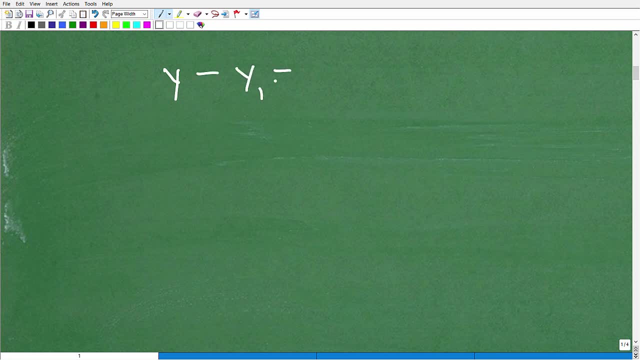 so let's write this now here: y minus y1, okay, All right, so here it is right. So let's say I'm going to use this little acronym here- find the equation of a line. okay, We already talked. 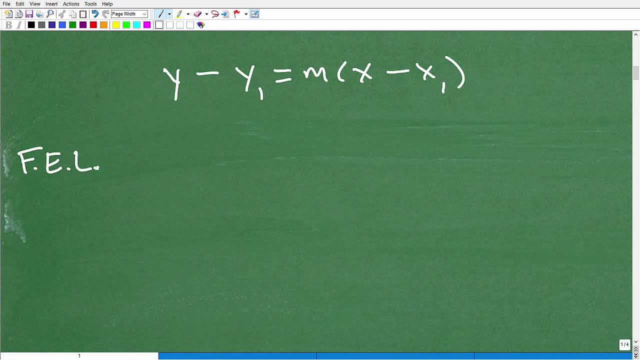 about what that meant. what we're trying to do here, right, We're trying to find the y equals mx plus b, so find the equation of a line that has a slope of, let's say, 3 and passes through the point. 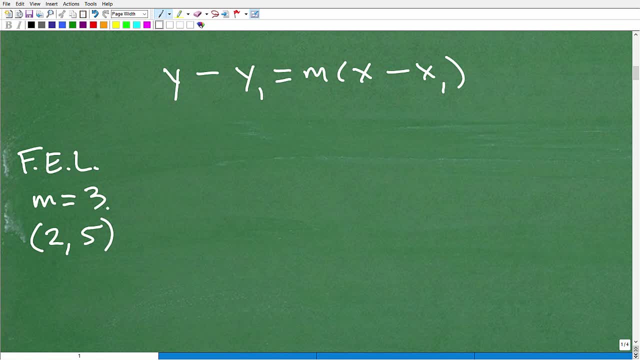 2, 5,. okay. So we have a line has a slope of 3, and it also passes through this point 2, 5,. so find the equation of a line. We're going to break out the point-slope formula, okay, So here. 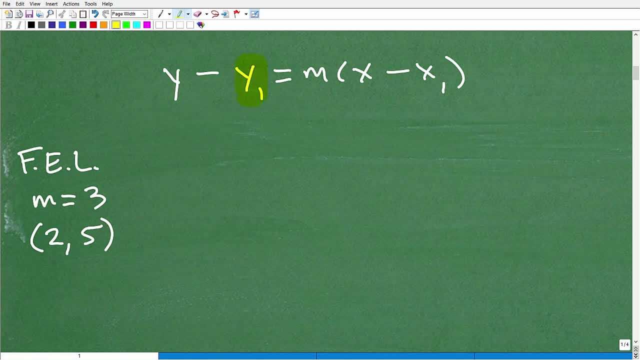 it is All right. so here's what you need to know: This little y1, this little m and this little y1- here are what we're going to be plugging in. okay, We're going to be plugging in values. 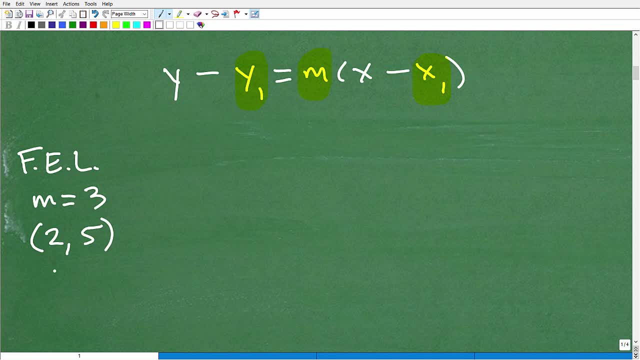 here: okay for y1,, m and x1.. So when we look at a point, okay, remember a coordinate. a point like this is an xy coordinate. It's a point all right. This first number here is going to be our x1,. 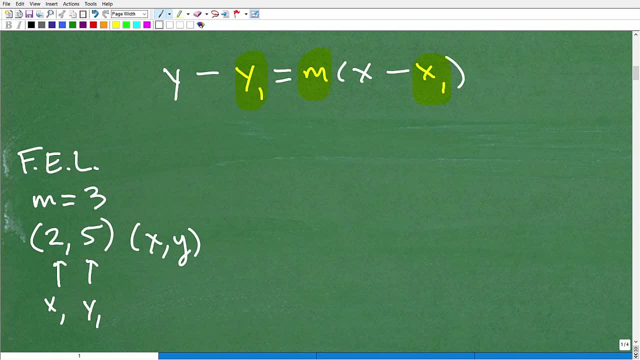 and this value over here is y1.. Of course we have m as 3,, okay, So don't let that confuse you all right with the x1, y1.. I know this kind of looks a little intimidating at first. 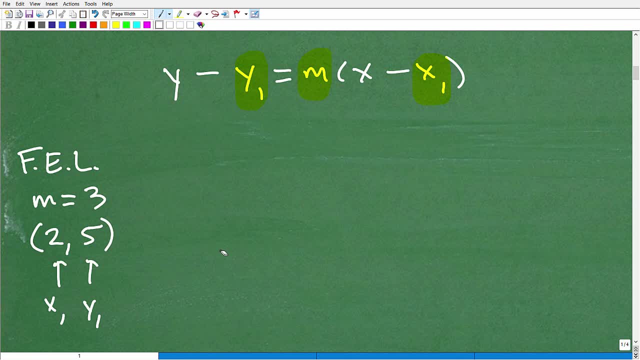 but it's really a very easy formula to apply. Okay, so let's go right to it and do this problem. Okay, so we're going to go ahead and first write the point-slope formula, okay, And then we're going to go y minus now using parentheses. we're going to be very careful because these could be. 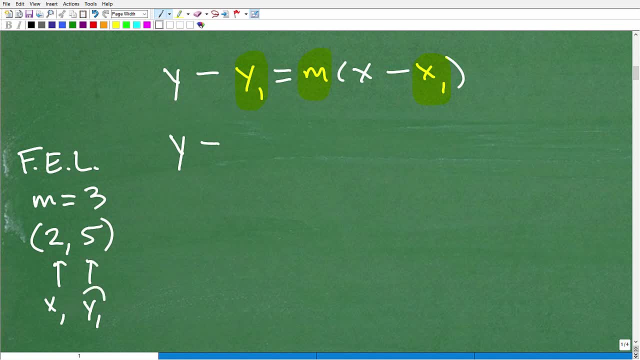 negative values, but we'll do another problem here in a second. So we're going to plug in y1, okay, So y1 is 5, so y minus 5 equals m, m is 3, okay, times x minus 2,. all right, And you can well. I always encourage you to use. 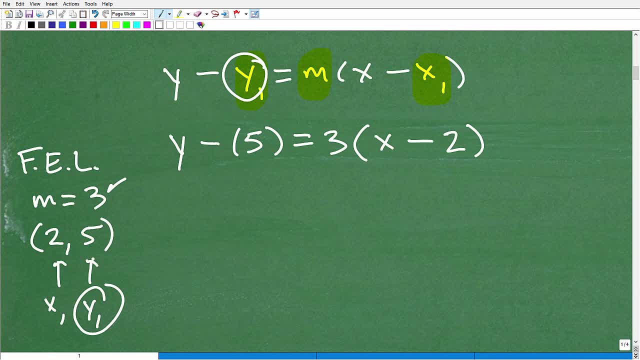 parentheses when you're plugging things in, especially with negative values. but if you're very careful, you could write it like so. okay, So here our x1 is 2, right, So make sure you understand how this gets set up. Once you understand the setup now, this is just basic. 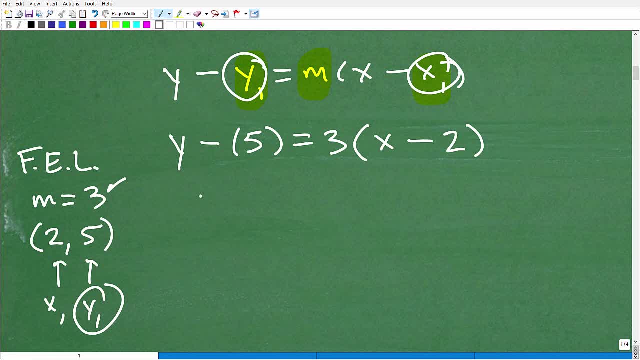 algebra. All right, so let's go ahead and clean this up and what we're going to be doing here for y? all right, And the steps are almost always the same, So it's going to be: y minus 5 is equal. 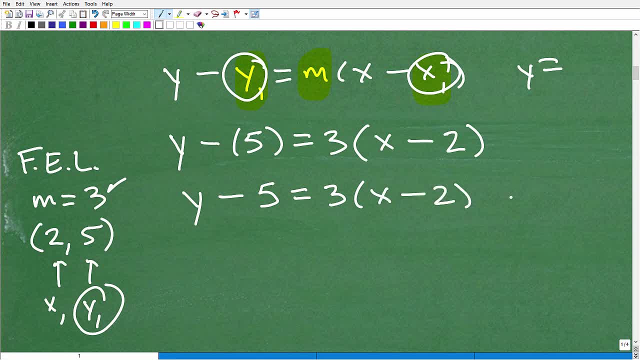 to 3 times x minus 2.. Now, right here is a place where students typically mess up, because this involves the distributive property. Our first step is: we're going to have to go like this and like this. okay, So this is going to be. y minus 5 equals 3 times x is 3x and 3 times 2 is 6,. 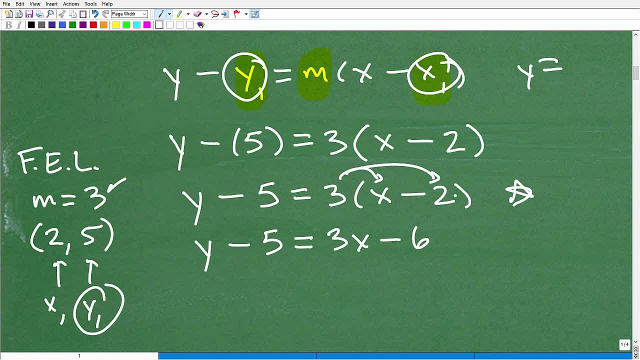 okay, or minus 6, all right. So the distributive property is a place where a lot of students make errors, so just be very careful that you correctly use the distributive property here and then to solve for y to get y. 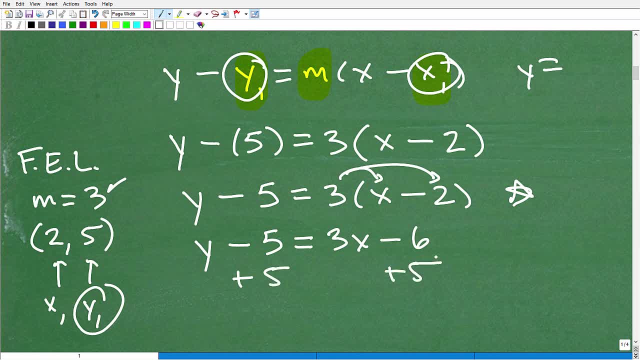 by itself. all I have to do is add 5 to both sides and just nice and neatly I can go. y equals 3x plus 1, and I am done okay. So y equals 3x plus 1 is the equation of a line, okay. 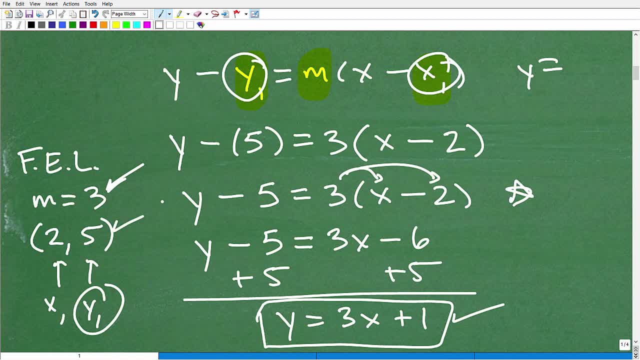 that has to be y, a slope of three, and passes to the point two, five. okay, all right. so that is illustration of using the slope at the slope intercept, the point slope. okay, there's a slope intercept and this is the point slope. okay, let's go ahead and 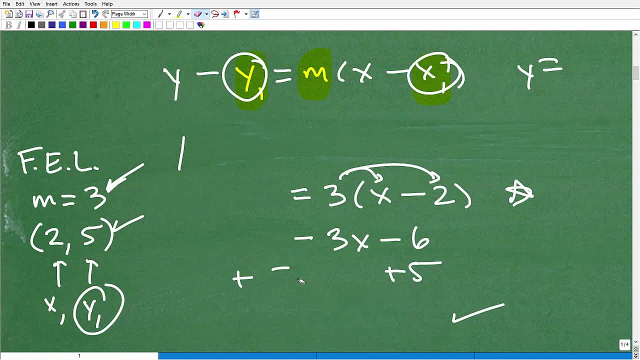 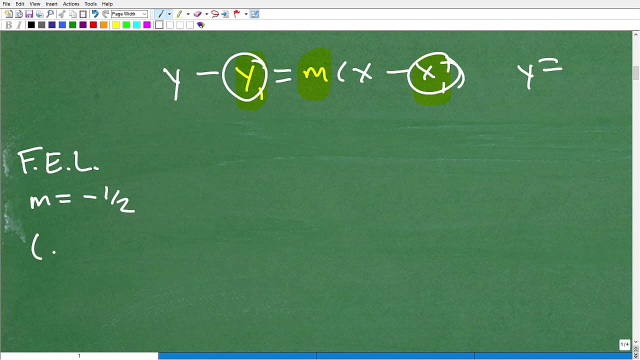 try another problem real quick, and then we'll wrap up this video, all right. so this time let's make it a little bit more interesting, okay, all right, so let's find the equation of a line where the slope is, let's say, negative one-half and the line passes through one negative four. okay, so if you want to pause the 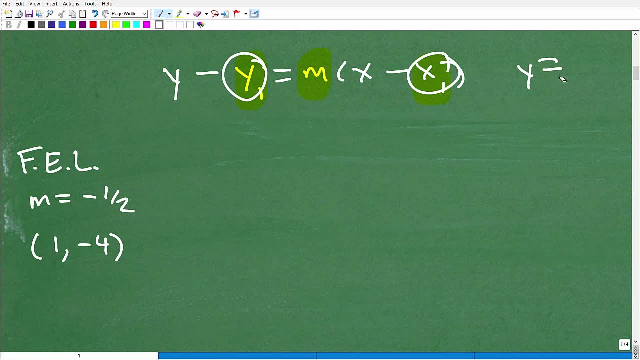 video. go ahead and see if you can do this problem on your own. all right, so let's go ahead and plug in the values. so Y minus Y 1- okay, it's going to be negative 4. now this is where you know you got a minus and you got a minus 4. 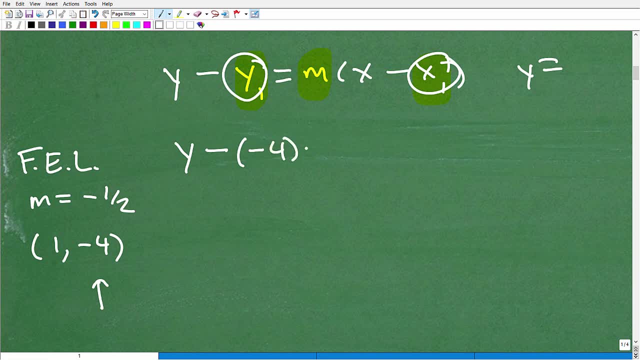 here for your value. so when you have these negative numbers you want to be using parentheses. so Y minus Y, 1- 2. just plug in the values first. don't try to do any any more additional steps. just plug in values first, like how we're doing here. okay, so Y minus a minus 4 M. 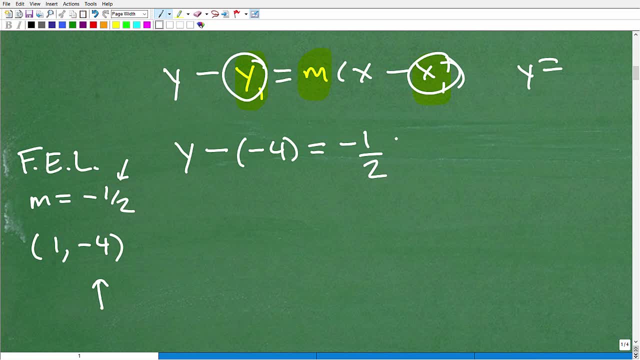 is negative 1, half, all right. X minus our X 1 is 1. okay, so double check that you plugged everything correctly. everything looks good. so at this point we want to start cleaning this up. okay, so we'll start over here. Y minus a minus 4 is: 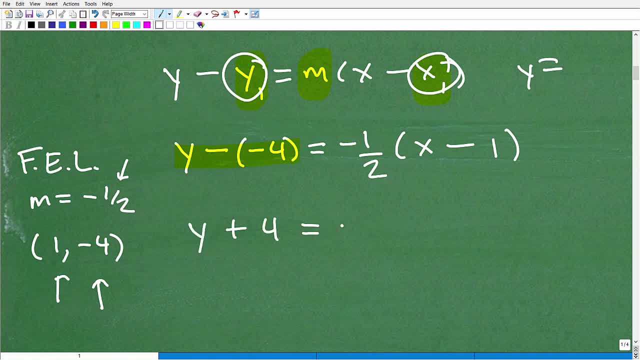 going to be: Y plus 4 equals negative one-half X minus 1. we'll just write it like so. okay, if we can kind of control and see that you know the steps in a one at a time. okay, at this point of the problem you want to go ahead and use the distributive property. 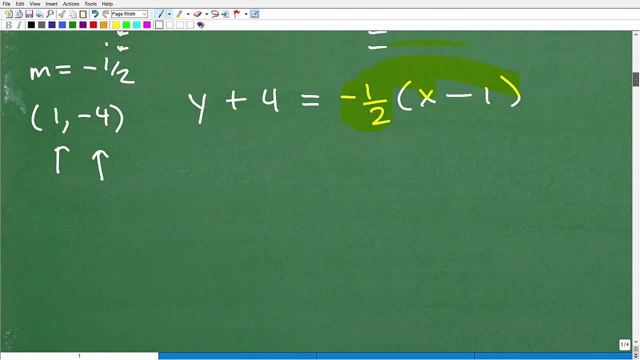 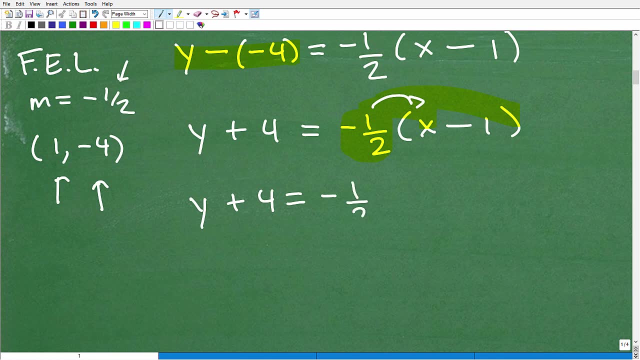 right here. all right, let's give ourselves some more room. all right, so this is gonna be: y plus four is equal to negative one-half times X, which is negative, one-half X, and the negative one-half times a negative one is going going to be what that's going to be? a positive one, half, okay. so negative times, negative that's.